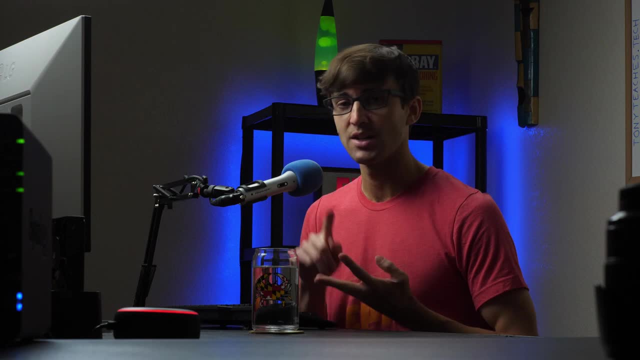 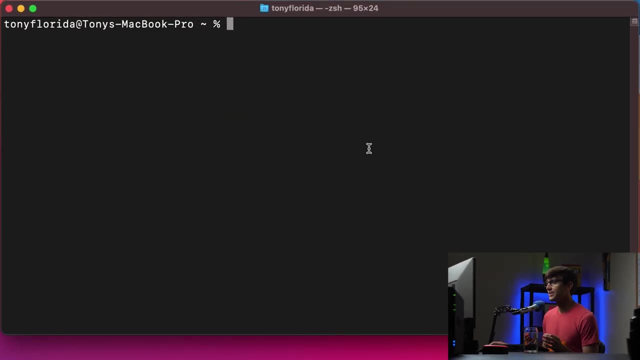 queries, some basic queries. as far as looking up, you know, A records, MX records, even reverse DNS records. So if that's something you want to learn how to do, let's go ahead and get on into the tutorial. here I'm going to be using my MacBook and by default, the dig command D-I-G is. 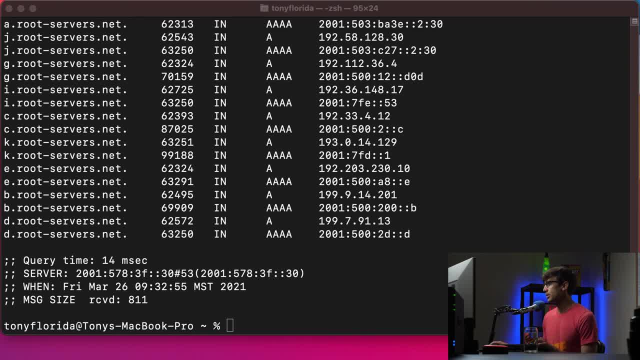 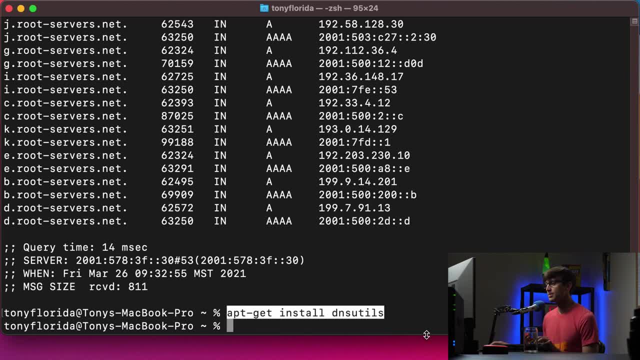 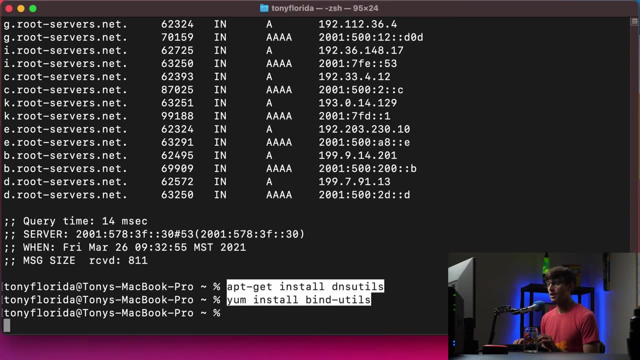 installed on Mac. But if you are, you know, on Ubuntu server or Debian server, you can install it with apt-get: install dns-utils And CentOS. it's very similar. yum install bind-utils- Okay, And then I don't. I honestly don't know about Windows. if there's a dig, 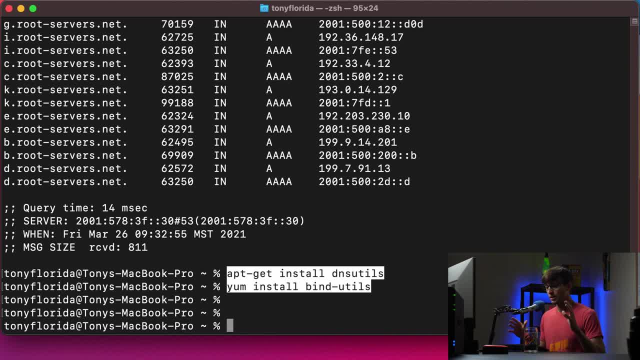 function in there. So I'm going to go ahead and install it, And then I'm going to go ahead and install it, And then I'm going to go ahead and install it, And then I'm going to go ahead and functionality on there. You'll have to do your own research. but if you're on Macs or a Unix type, 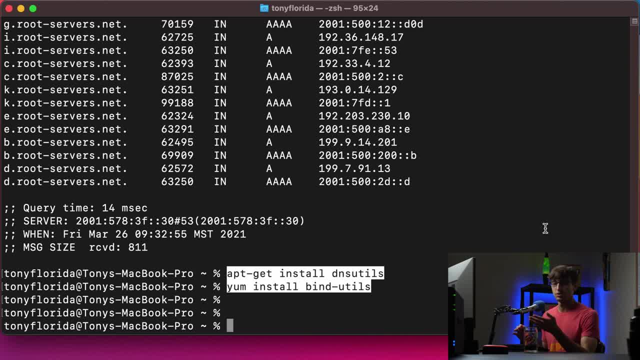 of operating system like that- Linux, something like that- then you should be good to go to follow along on this tutorial. Okay, So basically the syntax for a dig, like when you execute the dig command, you usually provide dig and then the name of the server and then the type of name. 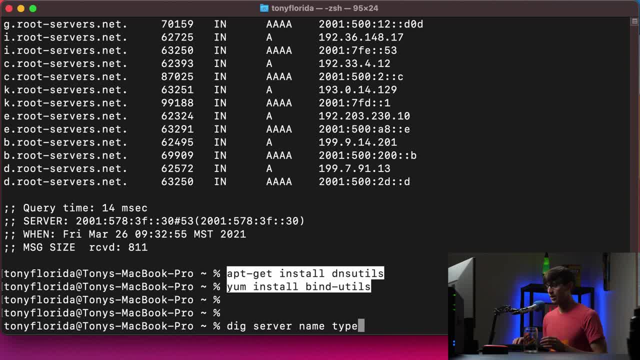 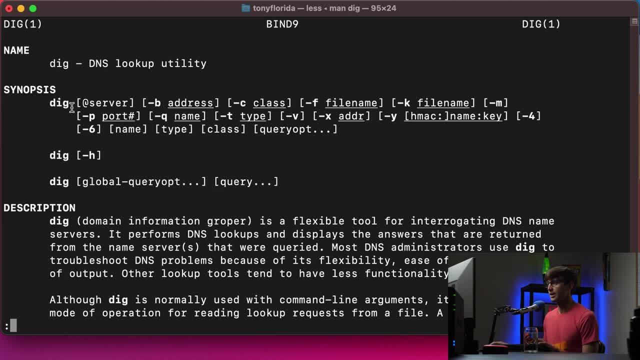 that you want to look up and then the type of record that you want to look up. So that's basically the basic syntax. And you can look at the manual for dig by typing in man, dig and you'll see that same type of information here. Okay, But let's go through some basic. 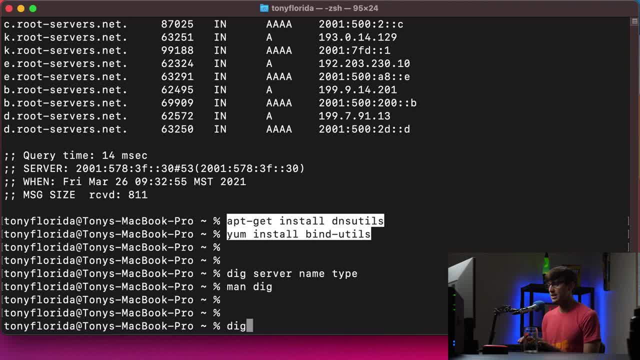 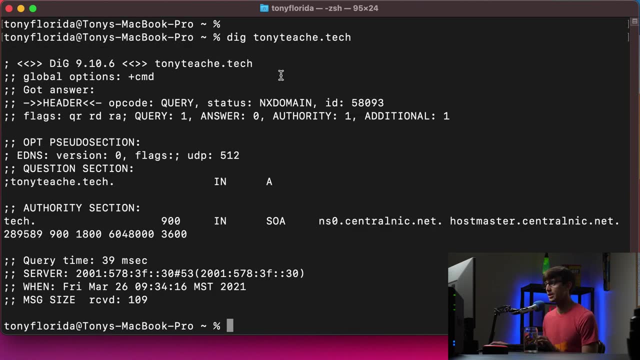 use cases here. So let's see, just if we do dig and then the name of a website, we'll use tonyteachestech as our example And by default, without specifying any of those options or any other command line arguments, we will look up A records only. So 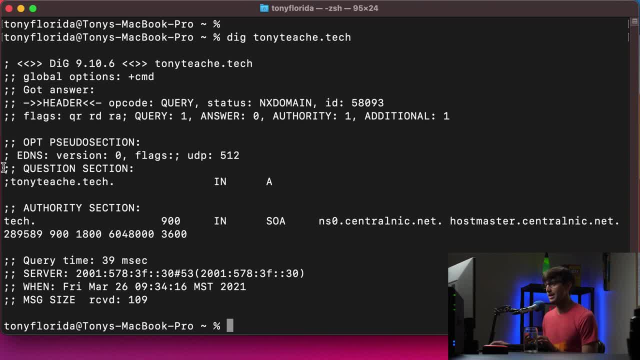 here. we can see that it's doing its thing here and it's spitting back out the A records for tonyteachestech And I spelled it wrong, So there is no A records. Tony teach, Yeah, I just need to. 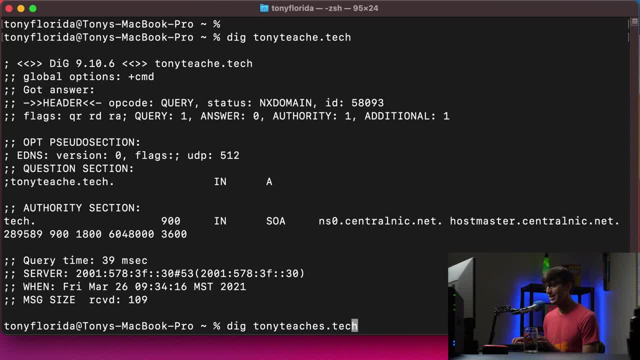 do that again, So tonyteachestech, And then we'll query that And there we go. This looks like more legit A records. So basically we have two A records here, one for this IP address and one for this IP address. Now, if that's equivalent right here as doing dig tonyteachestech A, we'll get back the. 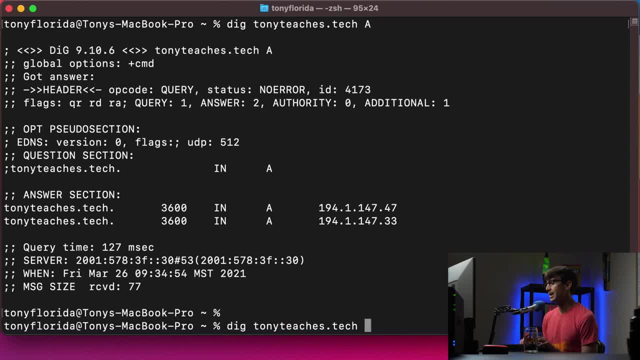 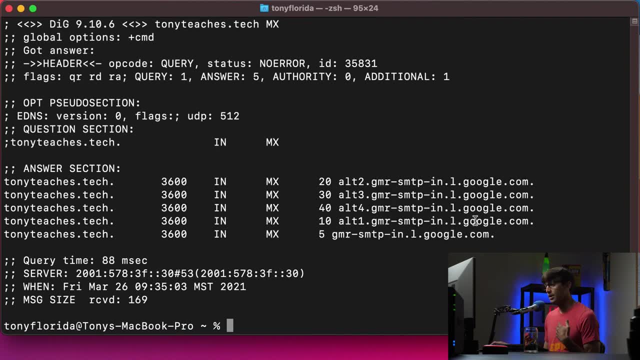 same exact thing. Now, instead of doing an A record, we can look up an MX record. So dig tonyteachestech and then MX, and that'll show all the MX records. So you can tell just by looking at this what type or, to a certain extent, what kind of email hosting I'm using And I'm using. 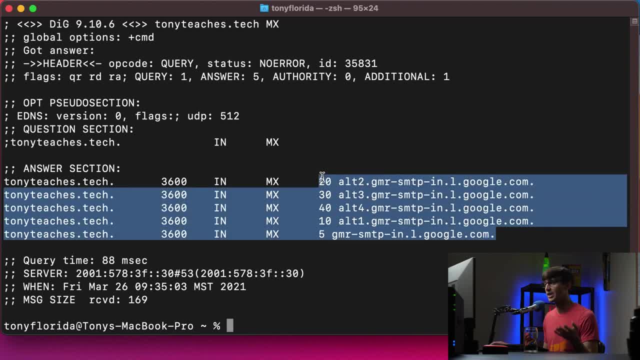 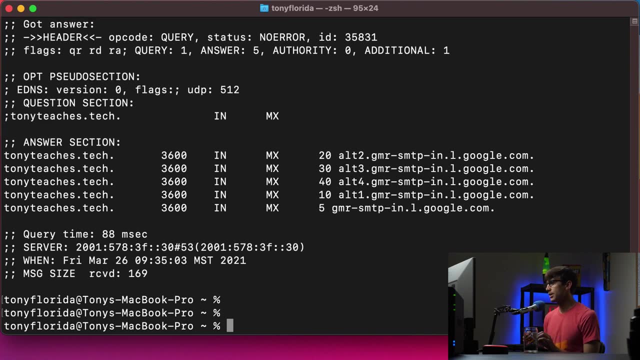 the Google's email forwarding email alias for my email hosting. So that gives you a little bit of insight there, because at the end of the day, all this information is public information. It's just a matter of knowing how to query it. You can also specify: 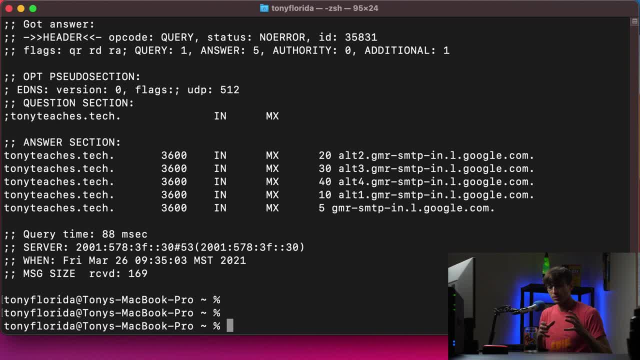 which DNS server you're looking at, because, as you know, or maybe you don't know- there's multiple DNS servers scattered throughout the world And, at all times, not all DNS servers have the same exact information. The information is being propagated from one server to the next with the 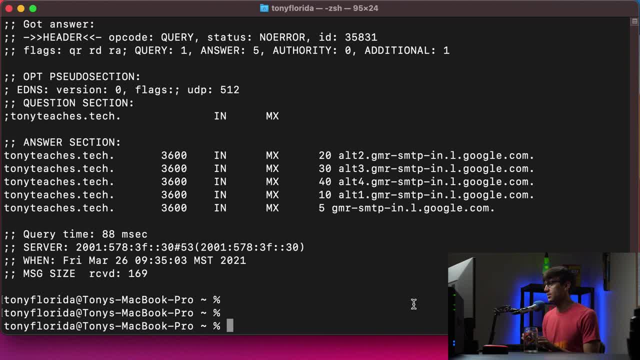 same exact information. So if you want to specify, for example, to use Google's DNS servers, you can do that with something like this: dig and then the at symbol and then the DNS server that you want to use. So if you're not familiar, Google owns the DNS server with IP address 8.8.8.8.. And then the: 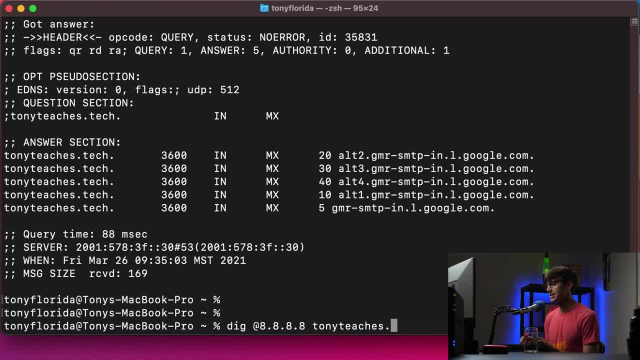 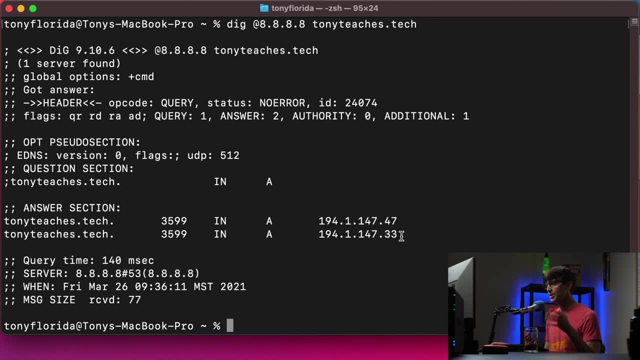 name of the website that you want to query. So again, we'll use tonyteachestech, And that'll, because it's the same, that'll return the same information, because the DNS servers are identical. Now, if we scroll back up here, I want to point this out. So the 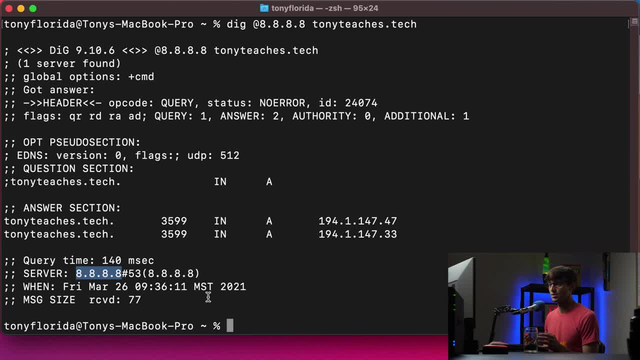 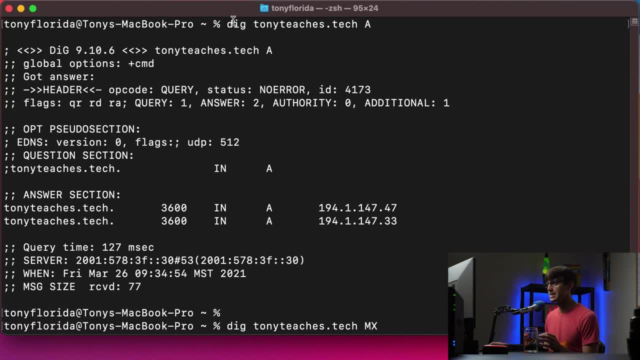 server at this point we're using is 8.8.8.8.. That's the server that we're querying. But if we go back up to when we did the dig without specifying the DNS server, this was querying this server with that, with the IP version six IP address. Where, where did this come from? Well, if, on your, if. 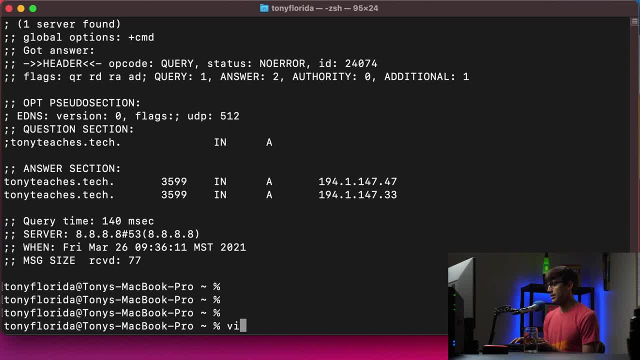 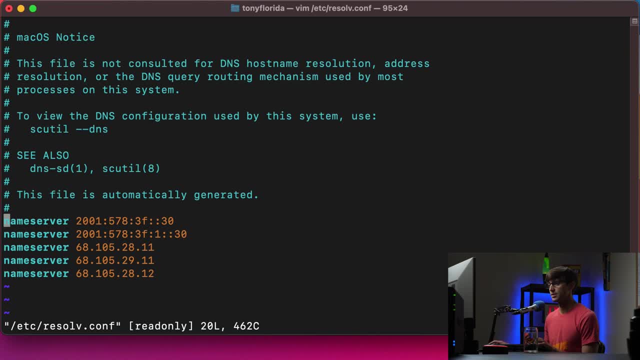 you're looking for a server that's similar for Ubuntu and Linux. if we look at our etc. resolvecom file, you'll see that these are the name servers that are preferred for our system. So if you wanted to, you can come in here and add in, you know, Google's name server if there's another. 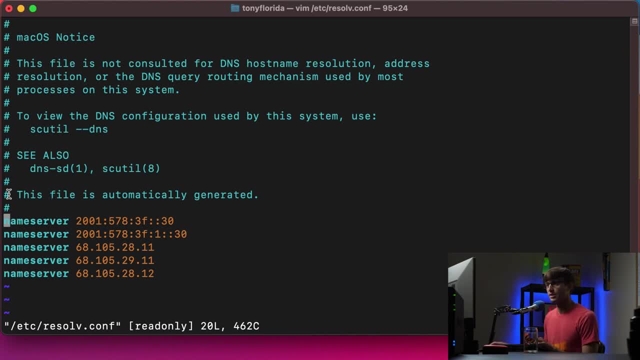 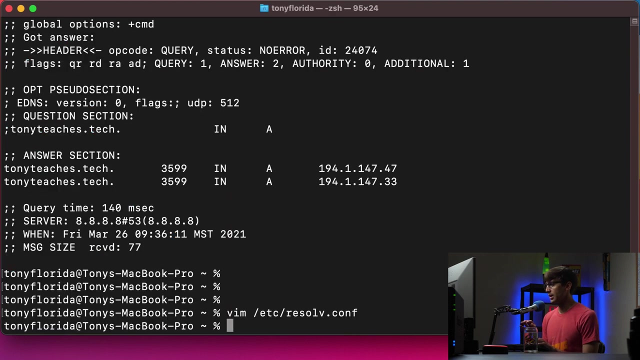 name server that you prefer, then you can add that to this. this file, Although this says this is automatically generated, So don't take my word on that, But this is. I'm just want to show you that that's where these are those name servers that our local computer is using. Okay, what if we wanted to see all the DNS? 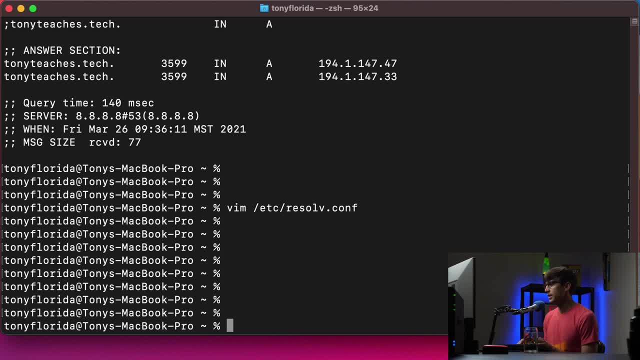 records for a particular domain name. Well, we can do that. We'll do that. We'll keep the same syntax. we'll query Google's DNS server, dig 8.8.8.8.. And then we'll say: Tony teaches that tech. 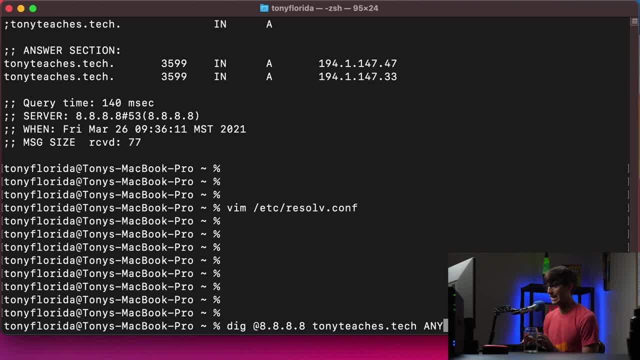 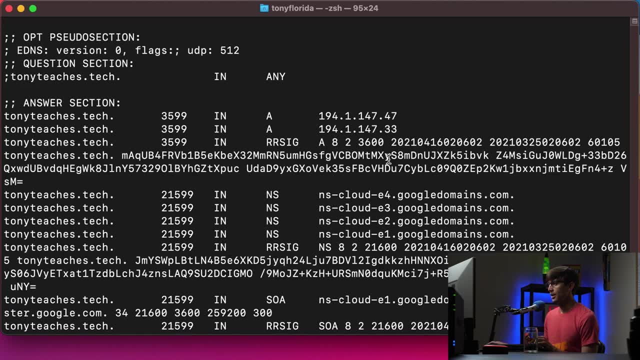 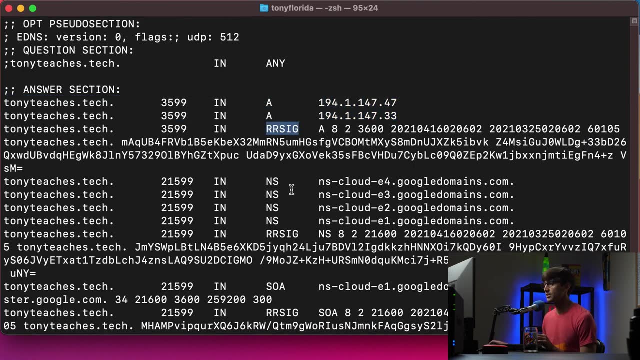 and then, instead of saying a specific record, we'll just say any, any DNS record for that domain name. we'll hit enter and we get a whole heck of a lot more information here So we can see the same a records. we can see. I'm not even sure what this is- our SIG and our 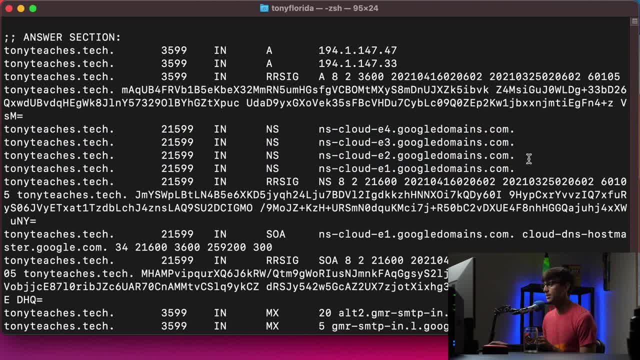 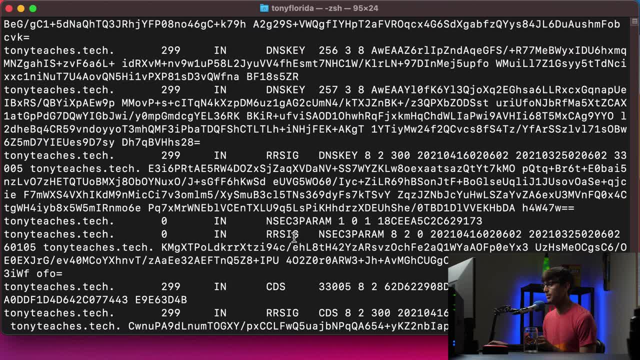 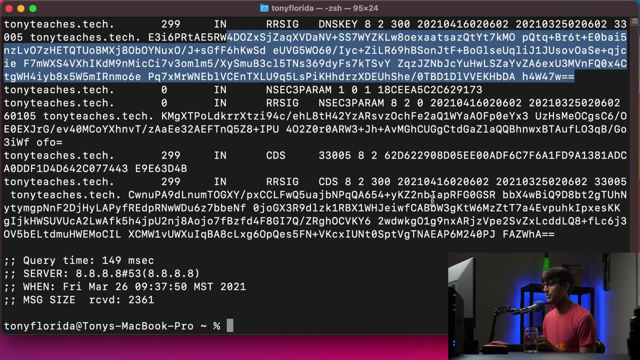 SIG record name server records. These are the name servers that I'm using, So a records those MX records. again, DNS keys: they're huge values like this whole thing. pretty much is the value. Yeah, so that's. that's a way, a quick way to see all the DNS records for a particular domain name. 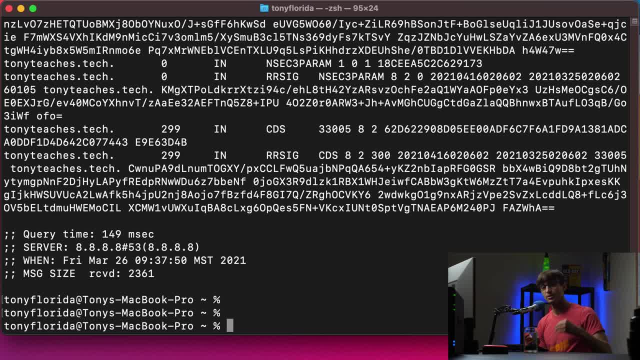 And, like I promised, we can also do reverse DNS. So how do we do a reverse DNS? And if you're not familiar, reverse DNS is a pointer record, PTR And instead of you know, an- A record mapping a domain name to an IP address. a pointer record maps an IP address to a domain name. So we already 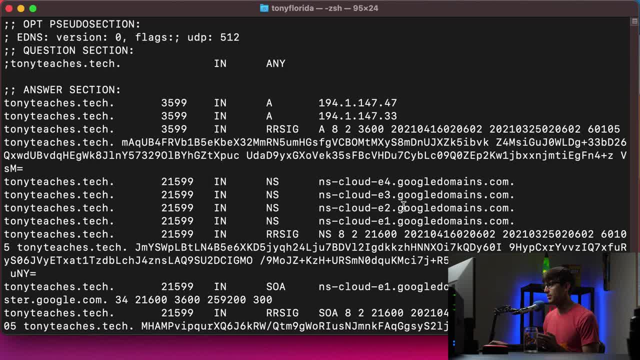 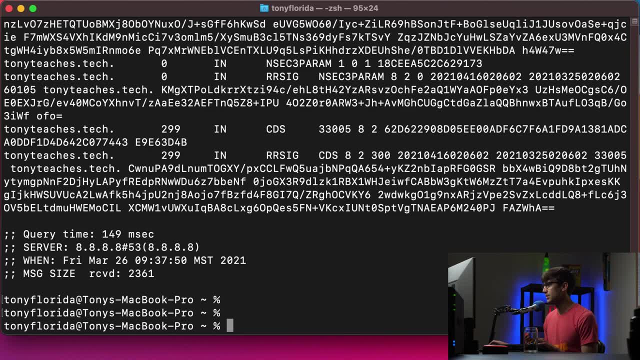 know the domain name for my website, Tony Florida, or yeah, Tony teaches tech. So let's use this IP address to see if we could do a reverse DNS lookup. So let's do dig And to do the reverse DNS lookup, you do dash x and then the IP. 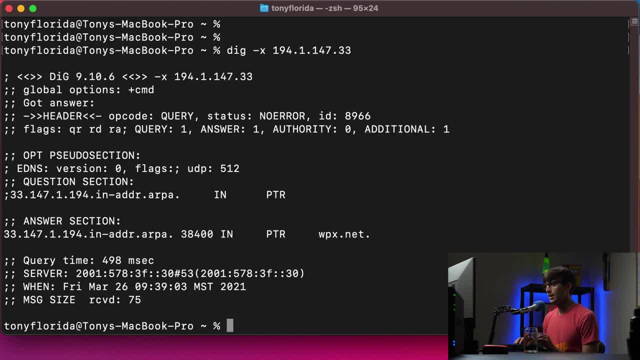 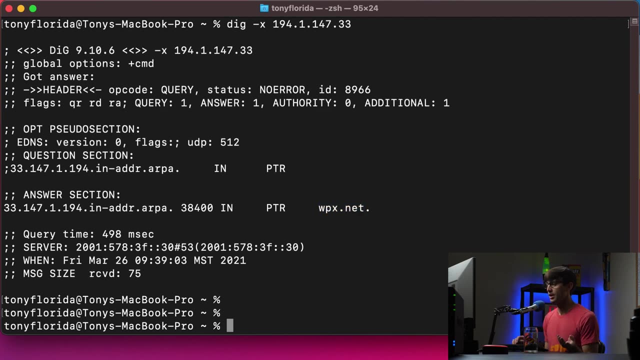 address, hit enter And you'll see. in this case, because I'm hosted with WPX, hosting WPX dot neck, that's what comes back for the value instead of my actual domain name. Now let me show you a different example. 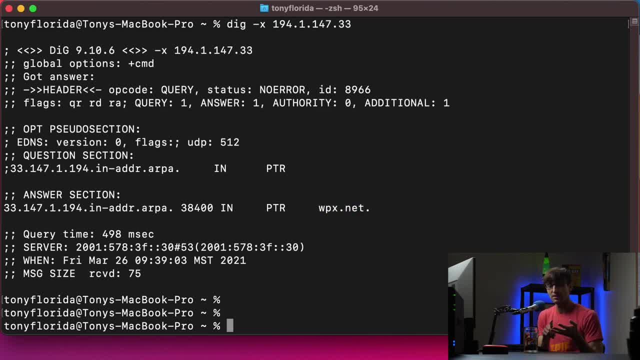 Where there's actually a one to one relationship between the A record and the pointer record, And I had set this up before. So I have a website called site six, dot, x, y, z. So we'll just look up the A record for that And you'll see. 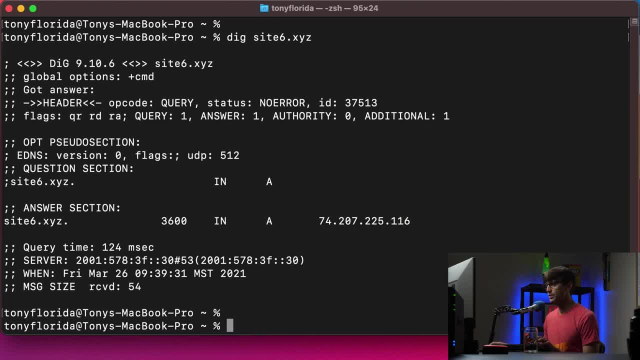 that, that's at this IP address. Now, if we do dig dash x and then this IP address, I have a pointer record set up for that And we should come back with the value of site six, dot, x, y, z, And there you can see the pointer record. 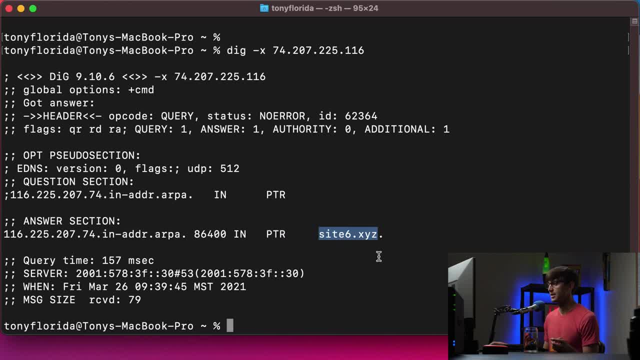 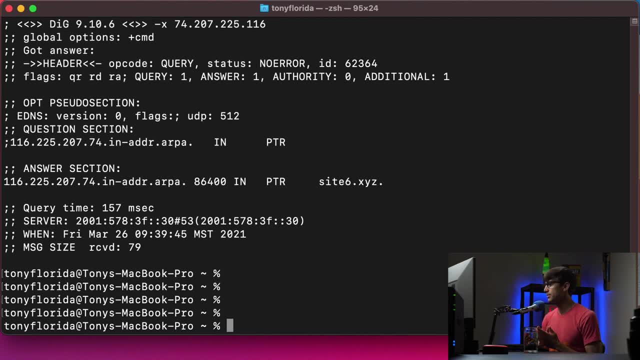 having a site six dot, x, y, z value as the actual value. This is this last part. the last thing that I want to talk about here is kind of related. It's still the dig command, but I just want to show you that this functionality. 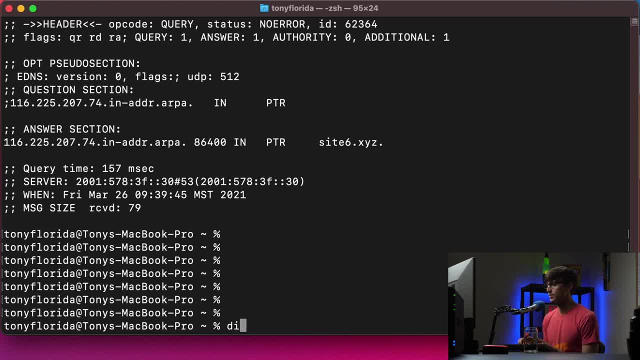 exists. So if we do, we can do a trace route with dig. So if we do dig, Tony teaches dot tech and then plus trace and this will go through all the servers that it hits on the web. So if we do dig, Tony teaches dot tech and then plus trace and this will go through all the servers that it hits on the web. 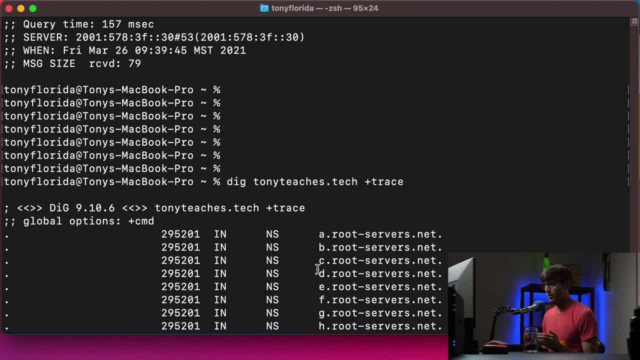 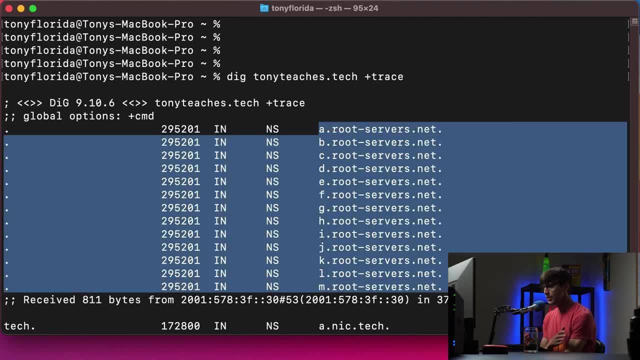 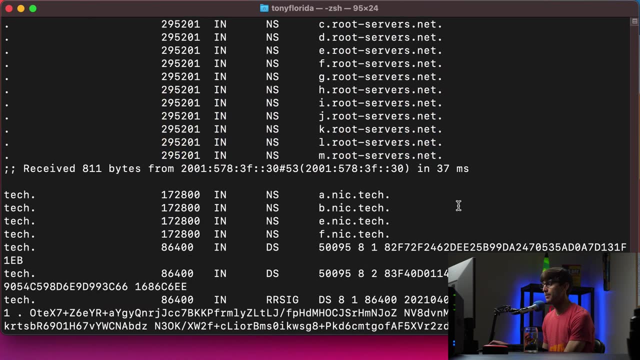 So if we do dig, Tony teaches dot tech, and then plus trace, and this will go through all the servers that it hits on the web. So what does that look like? Well, the first thing that it's going to hit is the root servers. Okay, so these are the root name servers. There's, I think, 13 of them, that kind of keep track of all the DNS records, And then it goes to the. 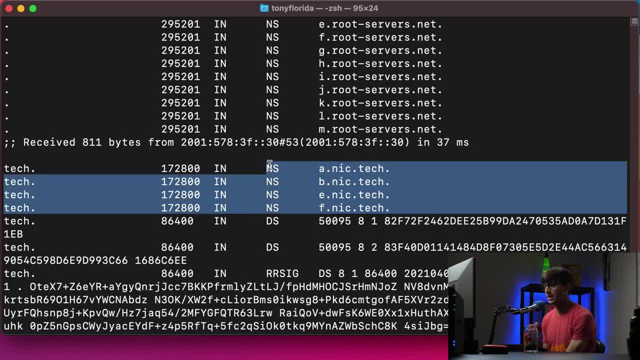 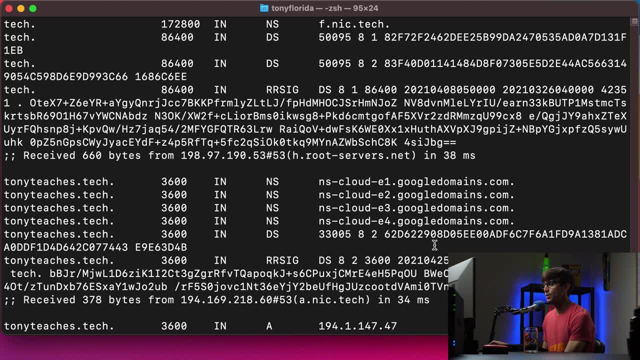 name servers that are specific to my domain name extension. So the dot tech domain name servers are next in this sequence, And then it goes to the root nameservers that are specific to my domain name extension. So the dot tech domain name servers are next in this sequence, And then it goes to, I guess, the spot r prompt. If we you don't tick it, currently it's your. 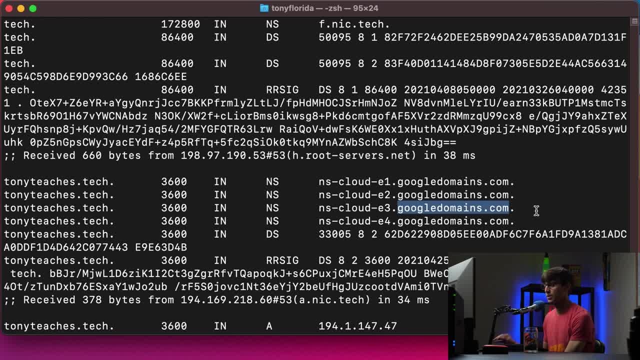 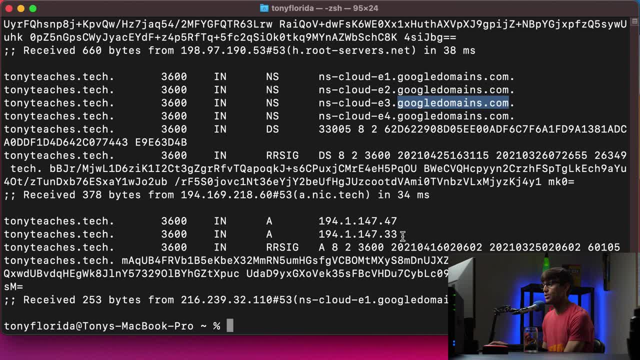 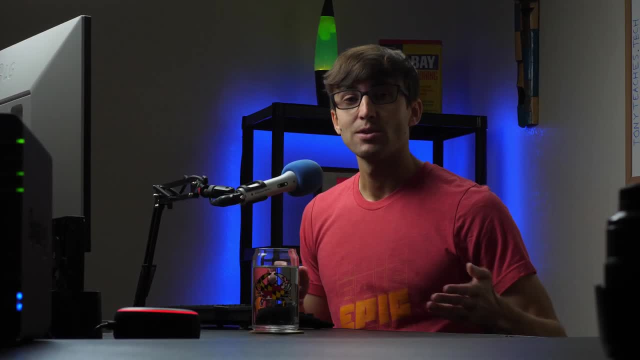 to Google's domain name servers, which are: I bought my tonyteachestech domain name from Google Domains, so that's next. and then, finally, it shows the A records for my domain name. okay, so that was a lot of information. hopefully made sense. hopefully you have a better idea about how to use the dig command to.